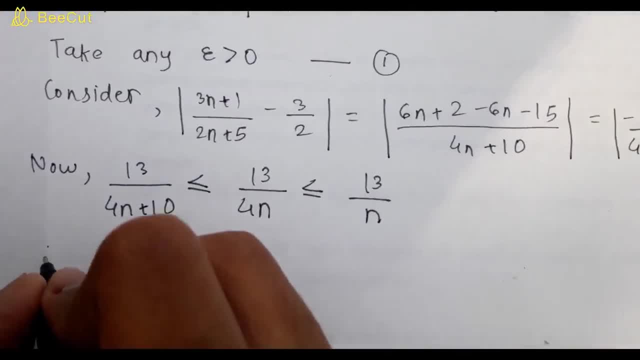 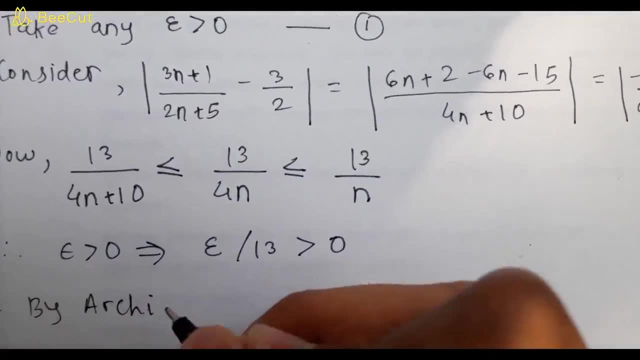 implies 1 upon n is less than epsilon by 13.. Therefore, epsilon is greater than 0, which implies epsilon by 13 is also greater than 0.. By the median property we can write: 13 upon n is less than epsilon by 13.. 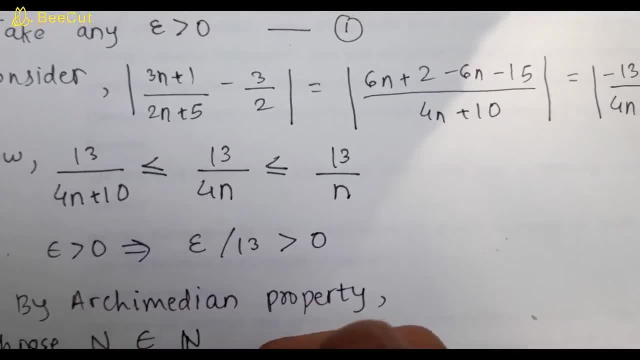 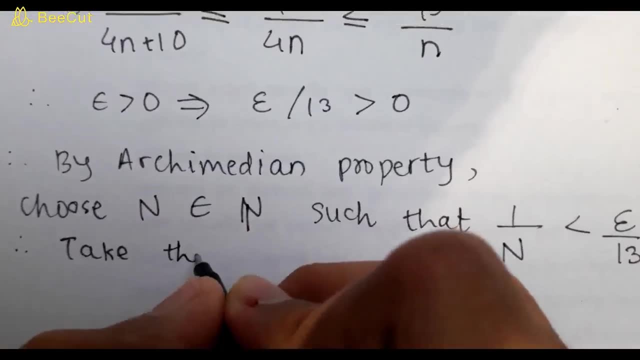 Choose capital. n belongs to natural numbers such that 1 upon n is less than epsilon by 13. Take this n and let mod of 3n plus 1 upon 2n plus 5 minus 3 by 2 is less than or equal. 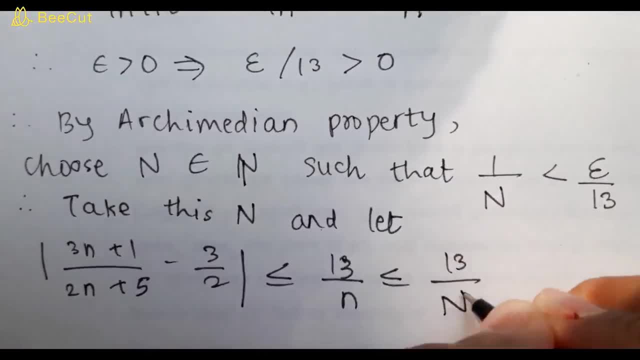 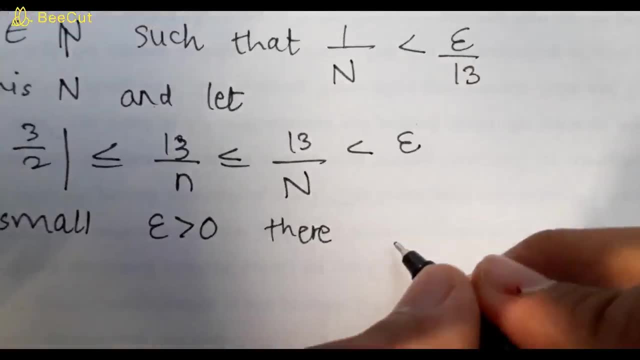 to 13. by small, n is less than or equal to 13. by capital, n is less than epsilon. For any small epsilon greater than 0, there are always n greater than or equal to n. So we can write стать to thisweis: exist a natural number, n, such that mod of 3n plus 1 upon 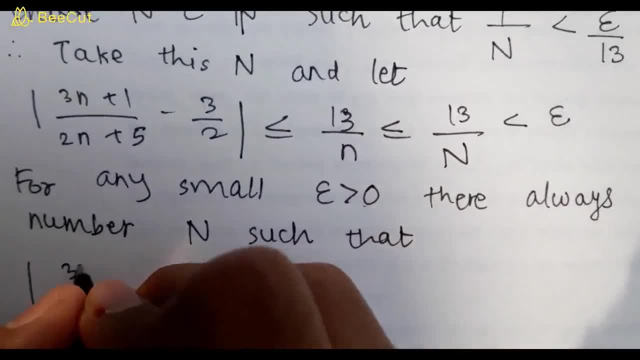 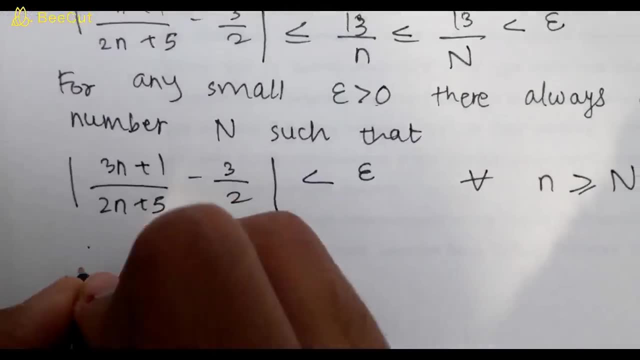 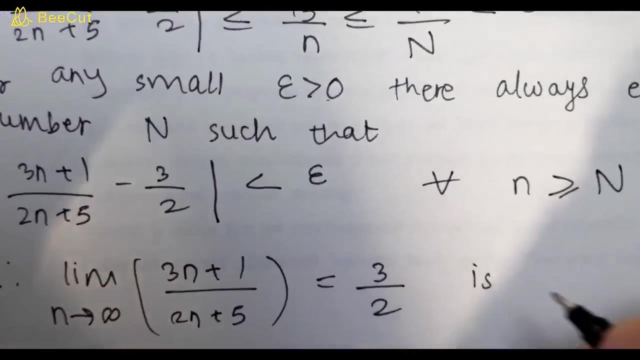 2n plus 5 minus 3 by 2 is less than epsilon for all n greater than or equal to n. Therefore limit n tends to infinity. 3n plus 1 upon 2n plus 5 is equal to 3 by 2 is proved. 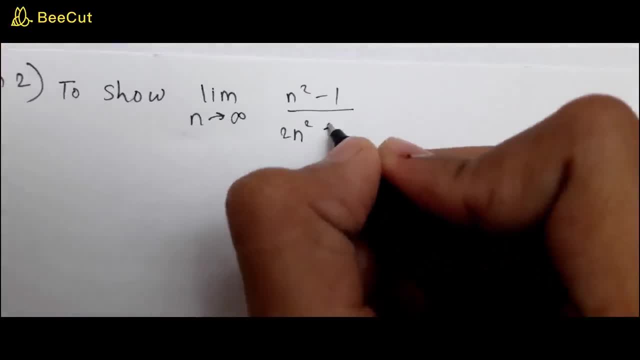 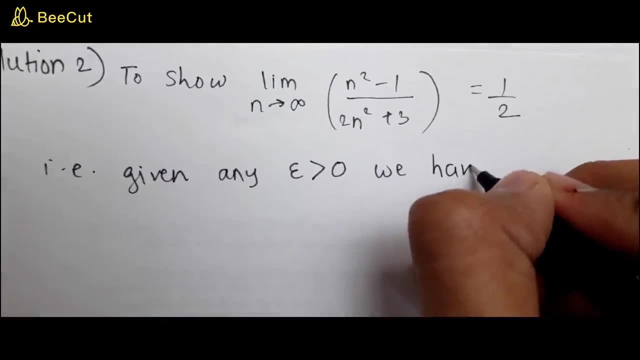 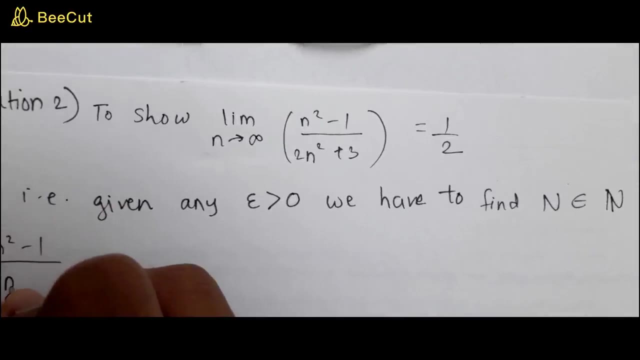 n tends to infinity. n square minus 1 upon 2n square plus 3 is equal to 1 by 2.. That is, given any epsilon greater than 0, we have to find capital. N belongs to natural numbers, such that mod of n square minus 1 upon 2n square plus 3 minus 1 by 2 is less than epsilon. 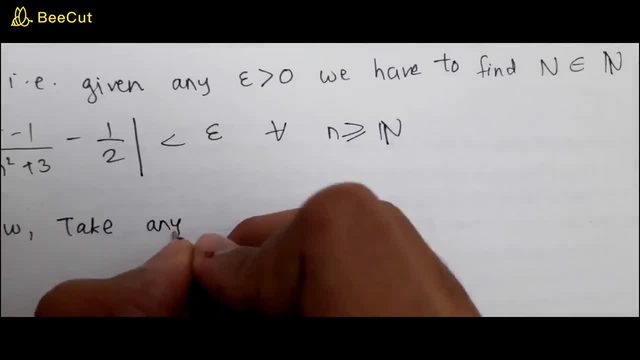 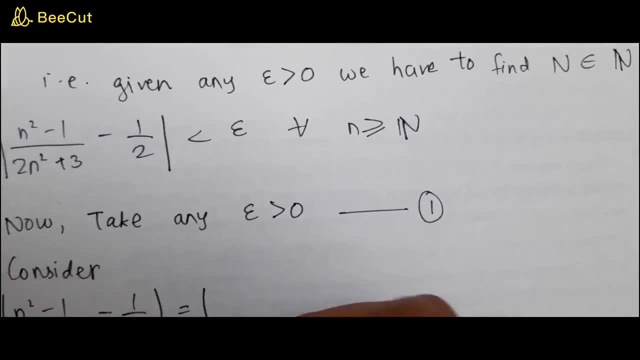 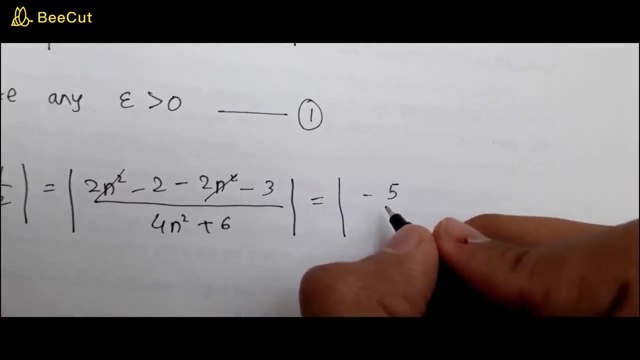 for all n greater than or equal to natural numbers. Take an epsilon greater than 0, consider n square minus 1 upon 2n square plus 3 minus 1 by 2. in mod On simplifying we get minus 5 upon 4n square plus 6, which can be also written as 5 upon 4n square, which is less. 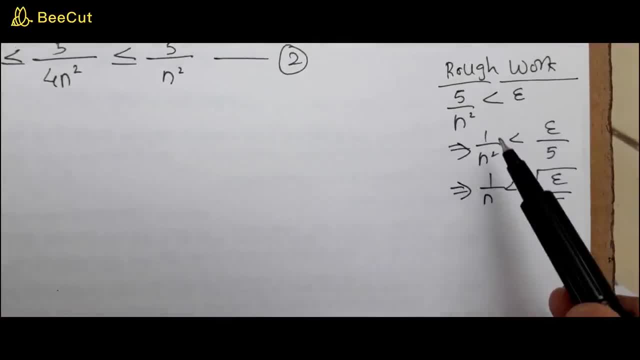 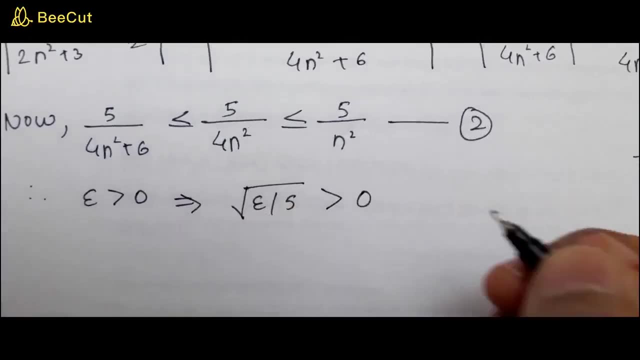 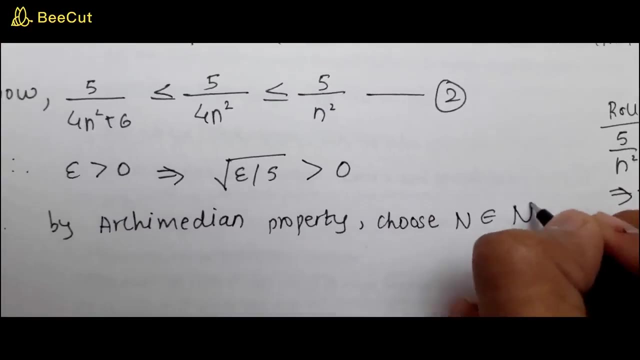 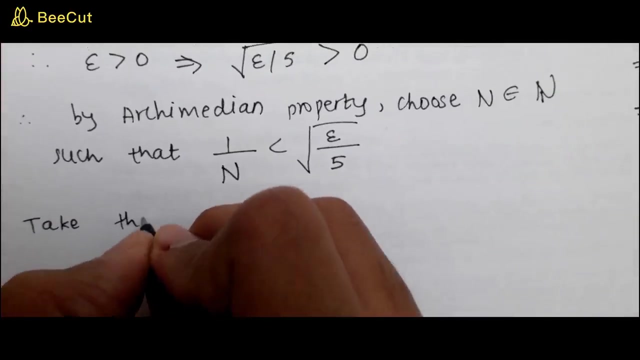 than or equal to 5n square. For doing the rough work. we can write as: 1 upon n is less than under root of epsilon by 5.. Therefore Barky median property choose n- belongs to natural numbers, Such that 1 upon n is less than under root of epsilon by 5.. Take this n and let mod of